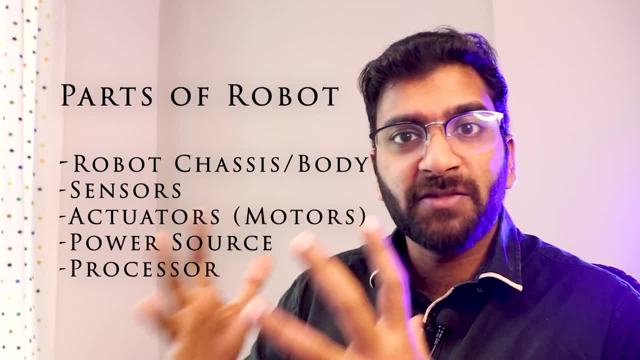 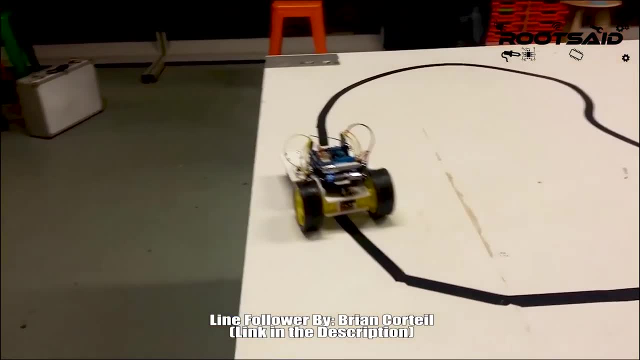 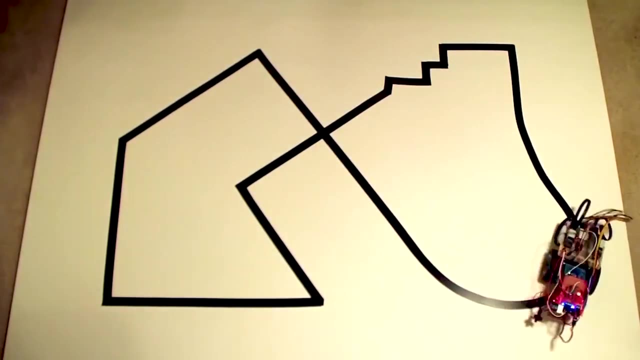 So let me ask you a question: Why do we need data from sensors? So that we can process it and do an output work right. For example, consider a line follower robot which will detect the line using IR sensors and turn on and off the motors depending on the sensor readings which will drive the robot. 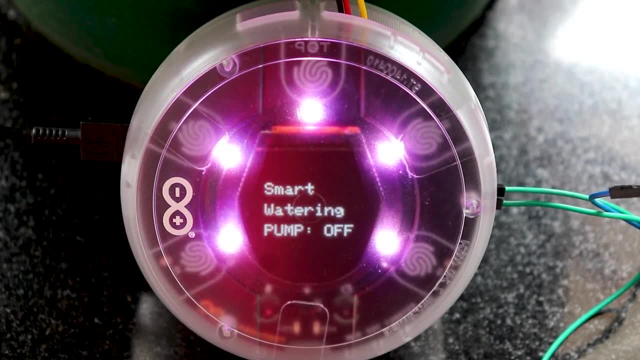 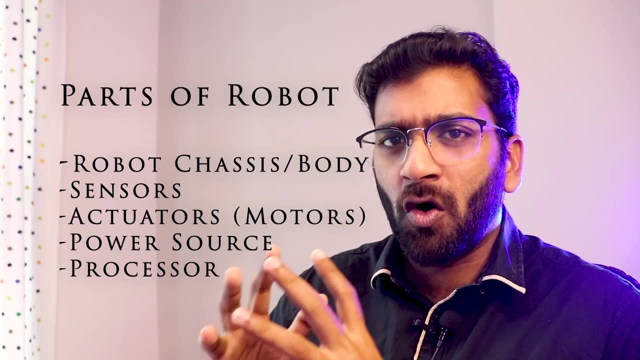 along the line. Or consider an automatic plant watering system Which will turn on the water pump when the moisture sensor detects the soil is dry. So the next question is: how do we turn on and off the motors or the pump, depending on the sensor readings? 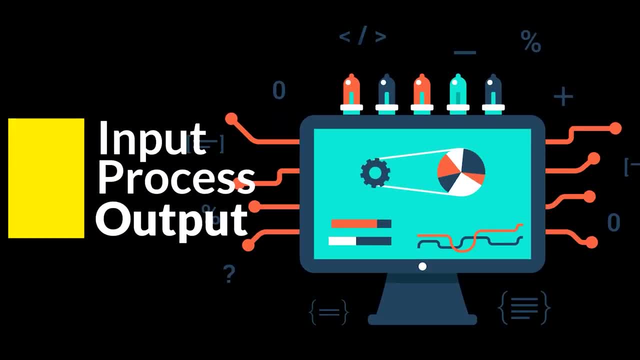 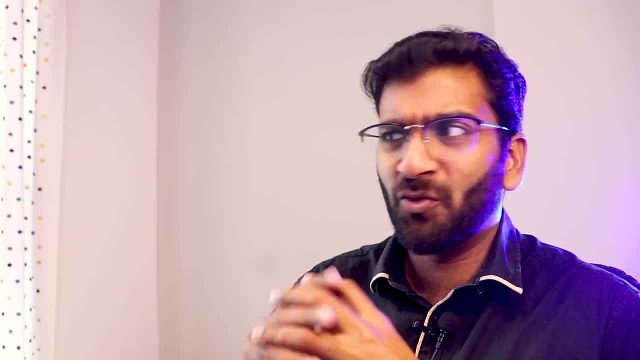 For that we will need a processing unit that will process the information and makes a decision. That's where Arduino comes to play. Let's see how we do that using Arduino. First, what is Arduino? Let me try to explain it in simple English. 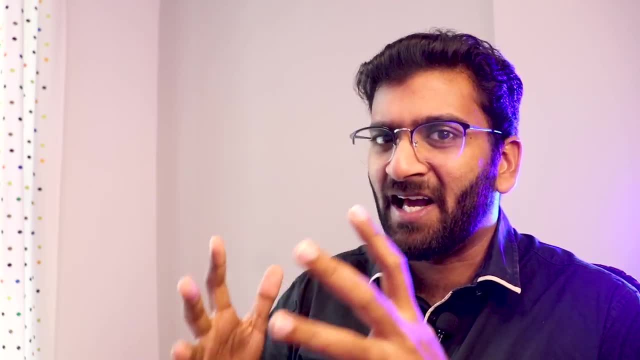 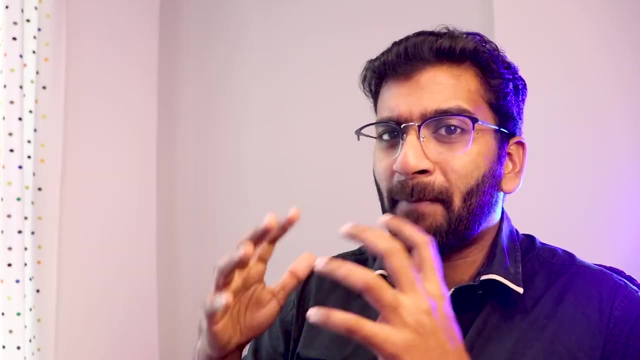 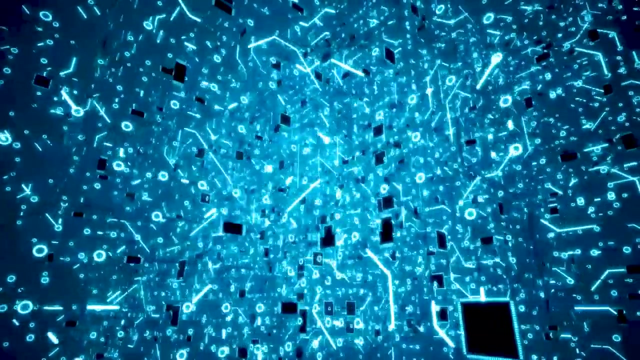 Arduino is simply a platform That will enable creators like us To create amazing electronics projects using simple coding techniques. But why is Arduino a platform? Because Arduino is not just a microcontroller board. Arduino comprises of three things. There is the physical board that uses the microcontroller, or the Arduino board. 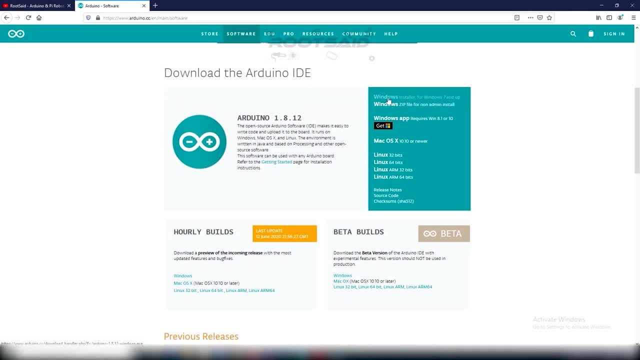 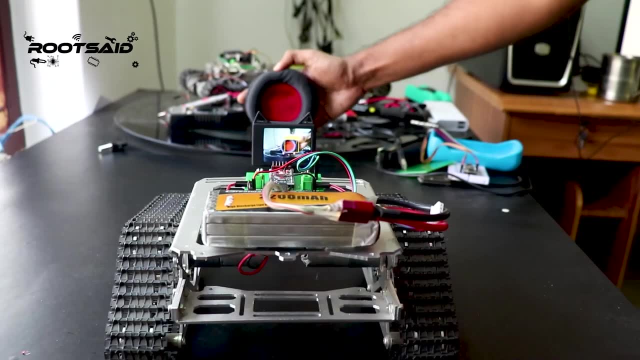 There is the Arduino development environment, called the Arduino IDE, And then there is the code itself, called an Arduino sketch, which gets loaded into the Arduino board. Those are the three components that basically make up what Arduino is. So let's see how we do that. 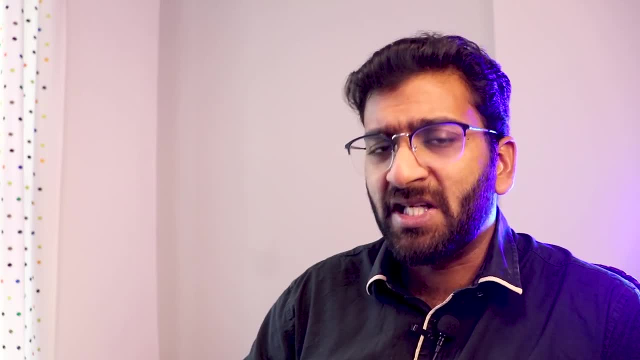 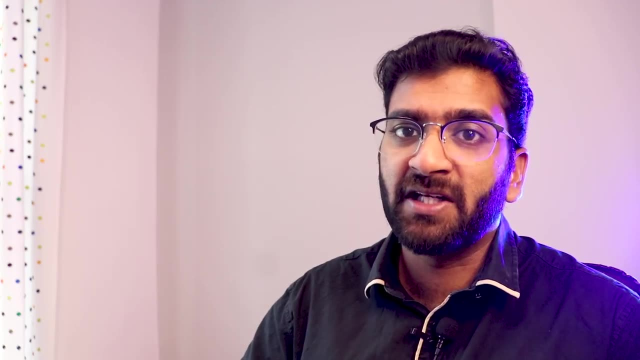 Arduino is open source. That means everything you need to make an Arduino, for example, the circuit diagram, the PCB files or the codes- are out there in the internet for free. You can either buy an Arduino board from the online market or, if you want, you can design. 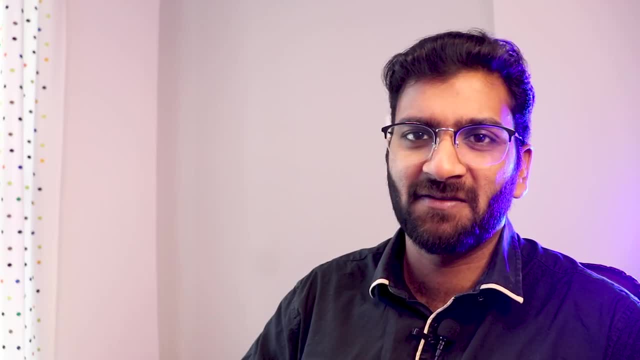 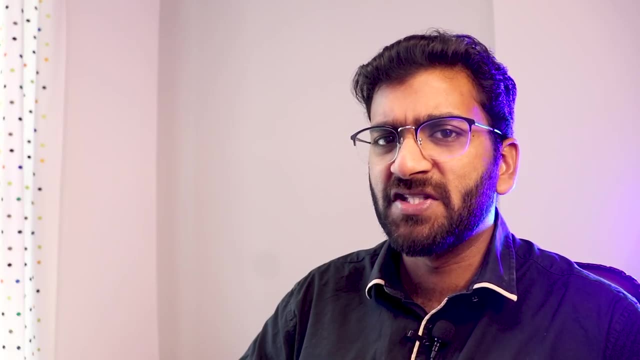 and create your own fully functional Arduino boards within minutes. You can use a breadboard to create your own Arduino or make a custom PCB, as I did in the previous video. In one of our previous videos, I showed you how you can create your own Arduino board. 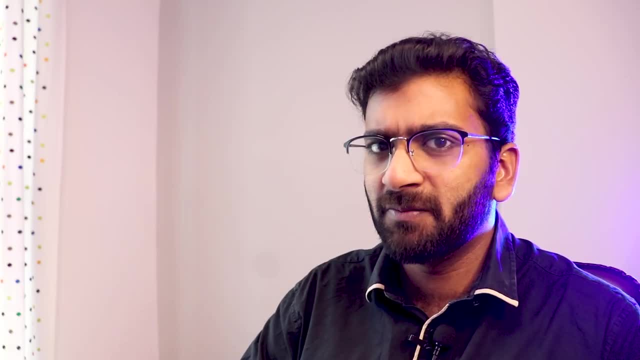 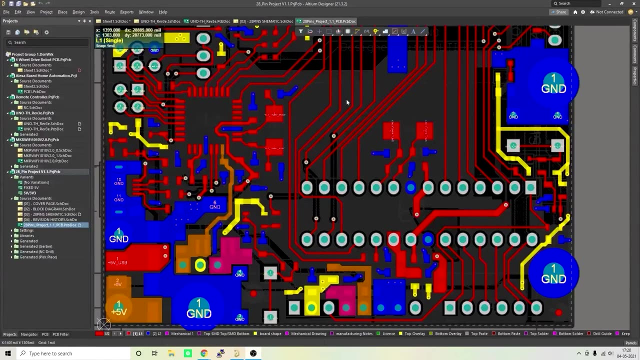 You can also use a breadboard to create your own Arduino or make a custom PCB, as I did in the previous video. You can use a breadboard to create your own Arduino board. I used Altium Designer to create my Arduino. Speaking of Altium, it's a powerful tool that can be used to design and create your own. 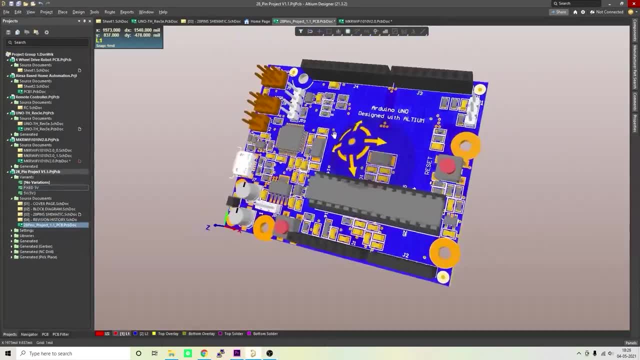 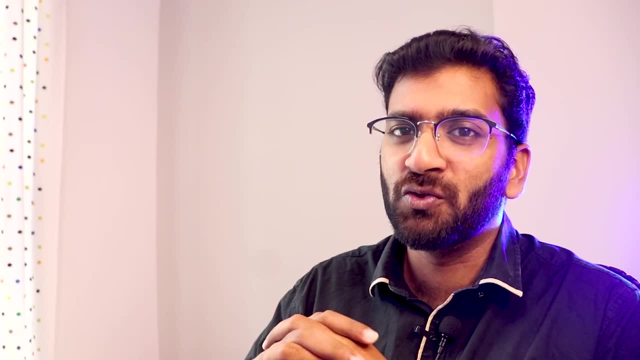 PCBs for your projects, as well as complex and multi-layer PCBs for industrial use. I have been using Altium Designer for the past three years and let me tell you guys, it's the best PCB designing tool I've ever used. If you're an electronics engineer, this is going to be really useful for you. 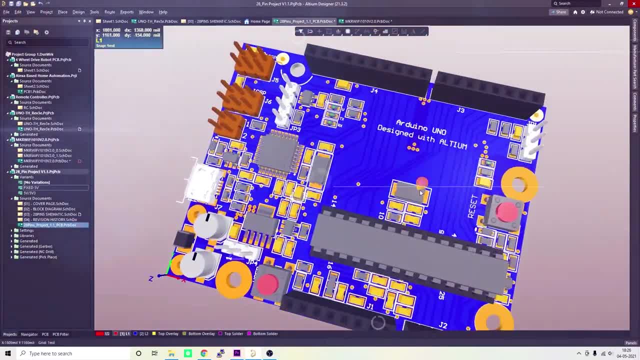 There are so many advanced features that enable us to create complex PCBs within minutes. I have been using Altium Designer for the past three years and let me tell you guys, this is the best PCB designing tool I have ever used. If you're an electronics engineer, this is going to be really useful for you. 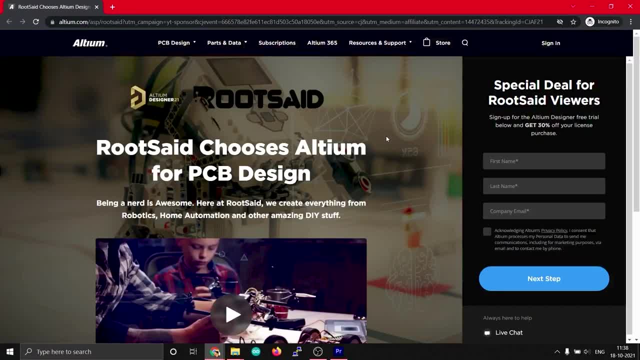 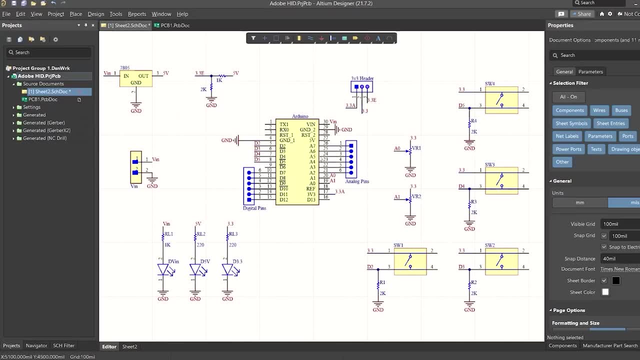 within minutes. I will leave the link to Altium trial version in the description. Make sure you try it. Also, there's a standing 30% discount for everyone who will be buying from the link below, So do make use of it. You will find a lot of PCB projects tutorials. 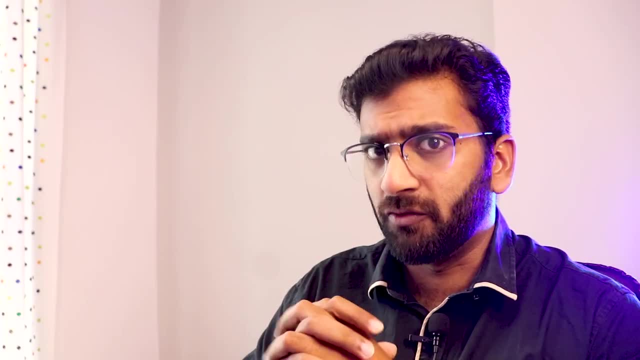 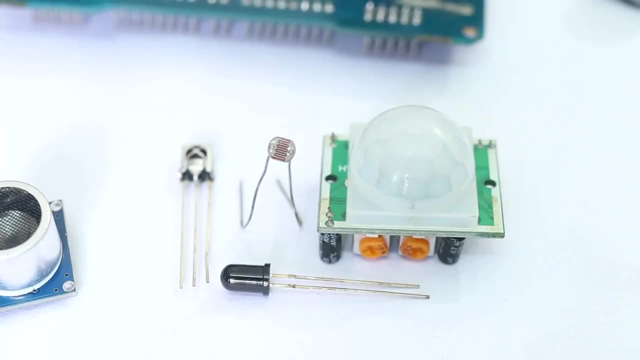 that we have done using Altium in our channel. How does Audino work? Now let's consider input and outputs of a robot. For inputs, you can think of sensors like temperature sensor, light sensor, touch sensor, flex sensor, humidity sensor, infrared. 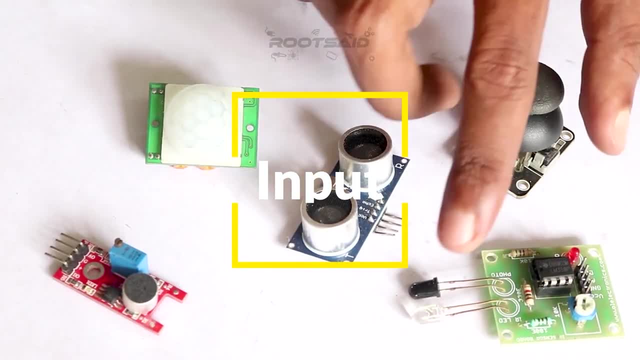 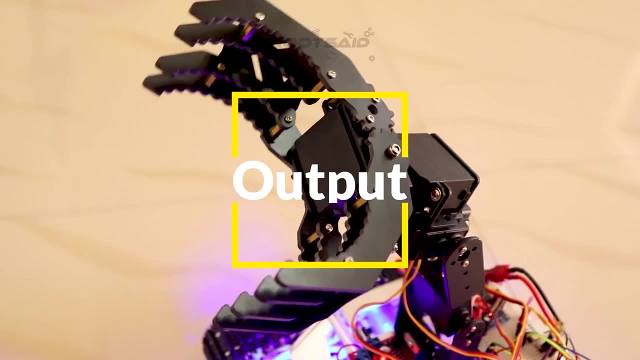 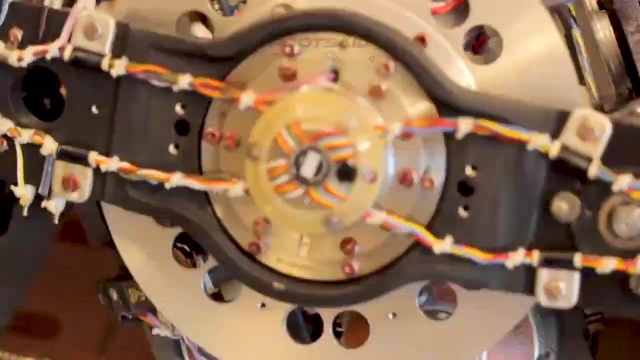 sensor, distance sensors and all those type of sensors can be read by this Audino board. Now, output would be things like motors, DC motors, servo motors, stepper motors, solenoids, LCD displays, LED indicator lights, speakers and electrical stuff that will do some type. 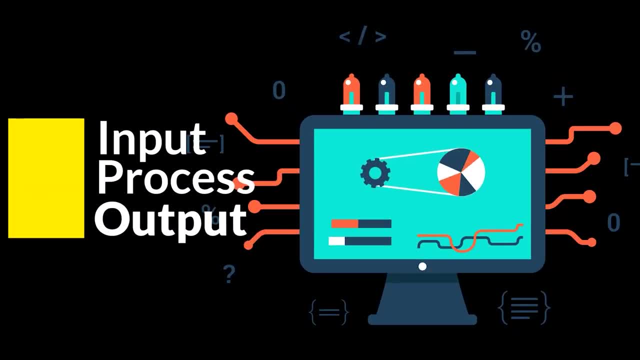 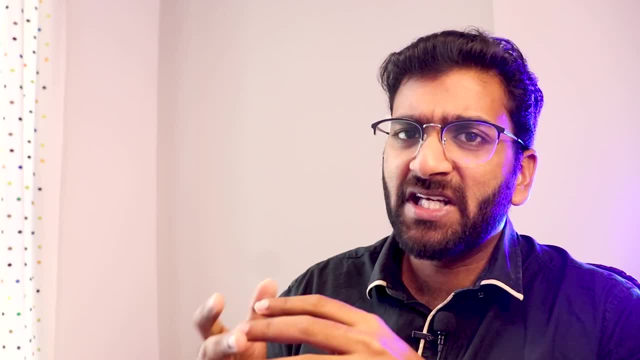 of action in the world Using Audino will be coordinating the input and the output. For example, if you want to control the temperature of your robot, you can control the temperature of your robot In Audino. we will write a condition like: if we get A as sensor reading. 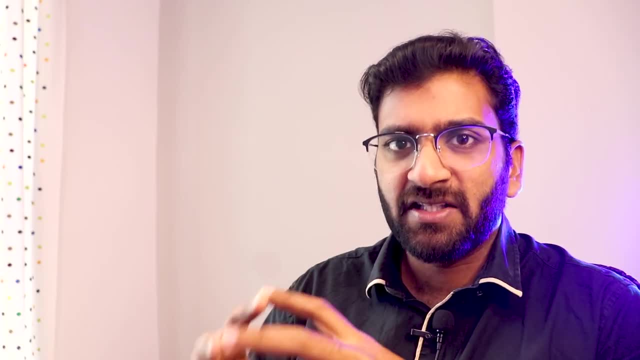 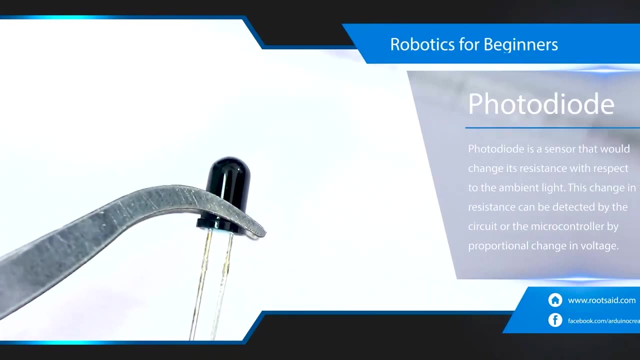 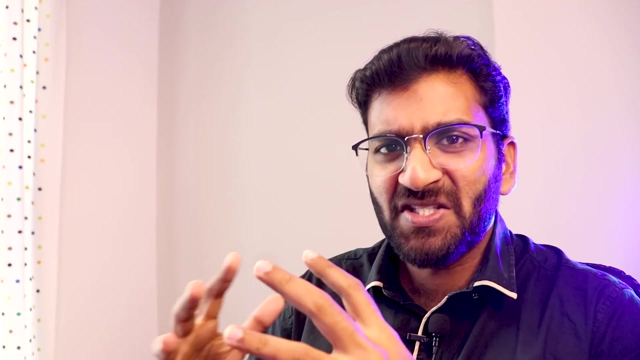 then do B as output. For example, let's connect a photodiode to one pin of the Arduino and an LED to another pin of Arduino. We can read the value of ambient light using the photodiode and write a condition to turn on LED when the ambient light is low. That is what we. 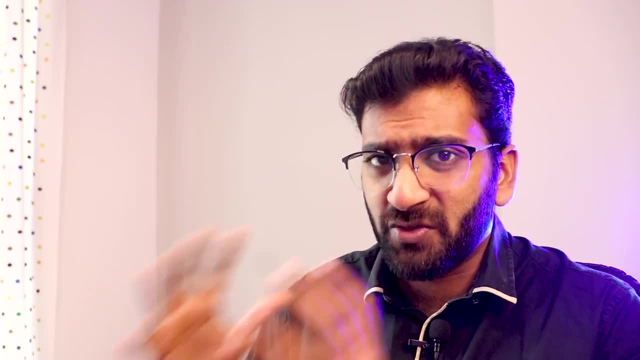 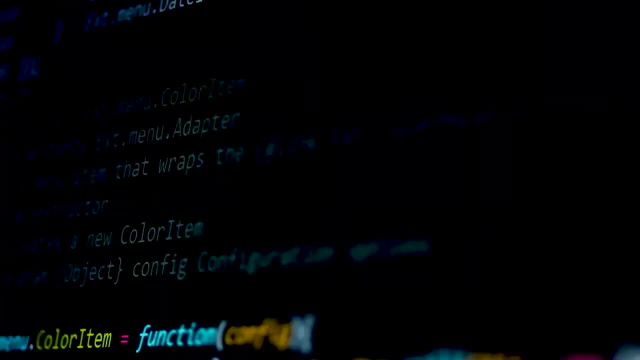 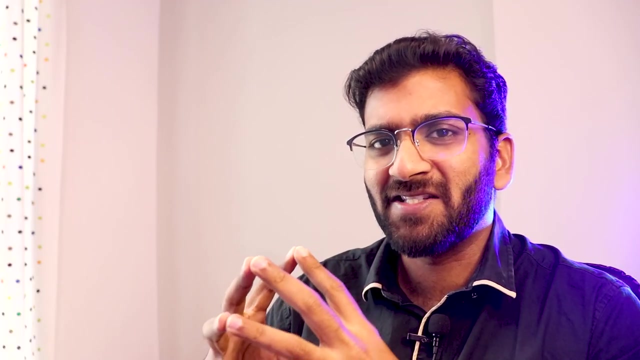 do with Audino. Now, there are so many microcontrollers out there that can do all this stuff, But why Audino? You know, microcontrollers have been quite difficult to use. One user guide is often over 300 pages long and it's jam-packed with technical lingo. But what Audino designers?